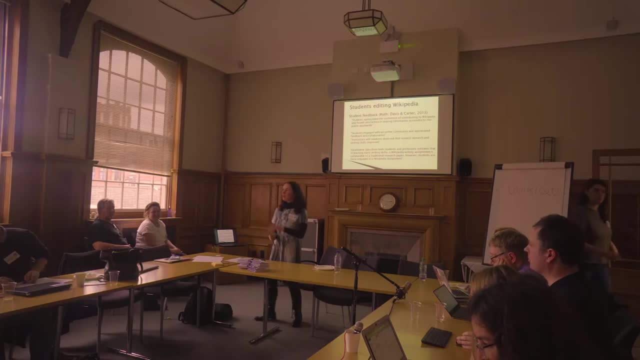 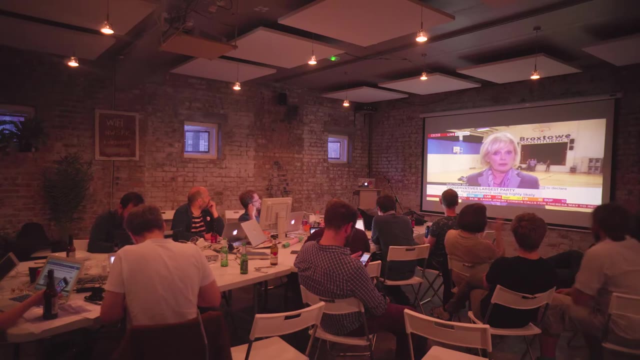 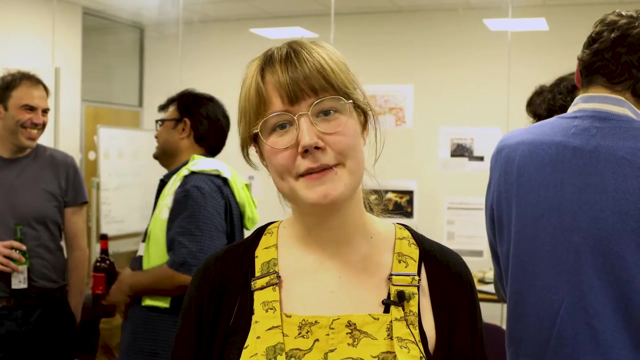 chapter for the global Wikimedia open knowledge movement. I joined Wikimedia in 2015, which coincided with the Wikimedia community starting to take the problem of gender inequality more seriously, with the launch of new initiatives such as Art and Feminism and Women in Red. Towards the end of 2015,, Wikimedia UK launched our own strategy for the period 2016-2019. 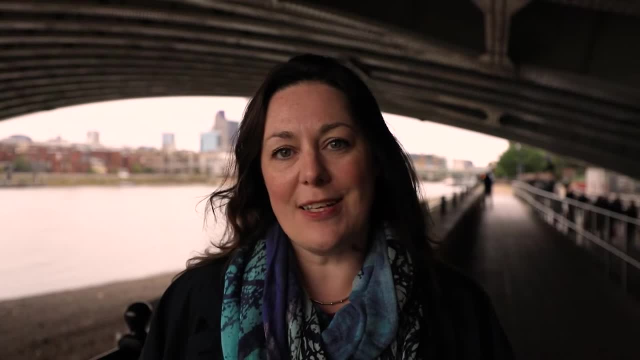 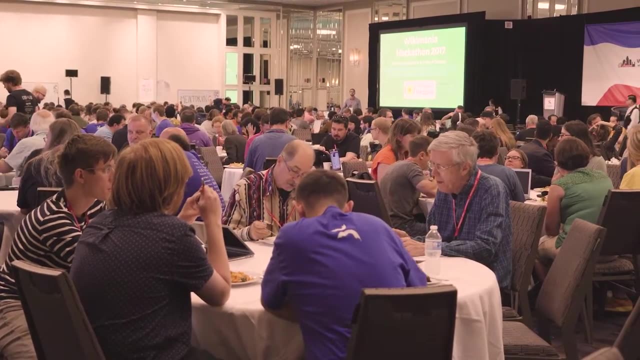 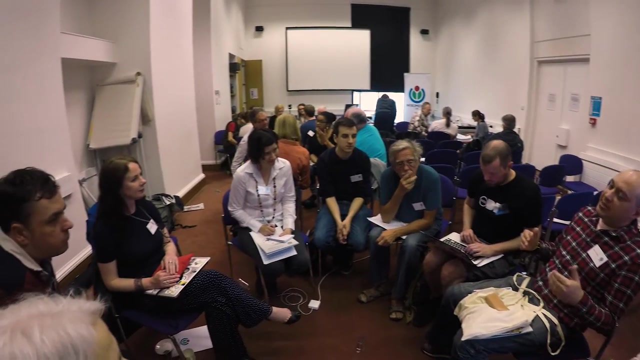 and at the heart of that strategy was a very bold ambition to eradicate inequality and bias on the Wikimedia project. One of our strategic aims for that period was therefore to increase the coverage of underrepresented subjects on Wikipedia and to diversify its content and contributors. 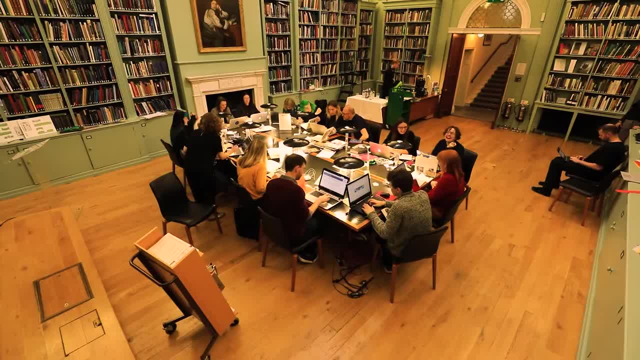 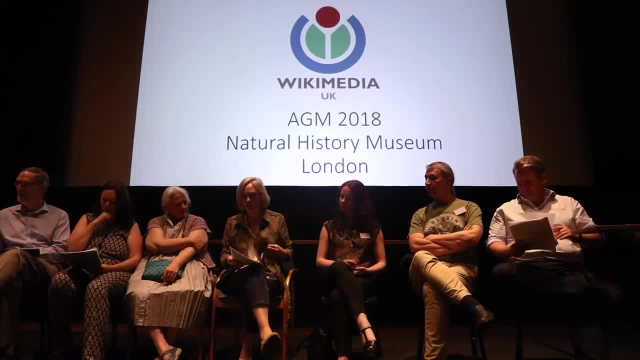 At Wikimedia UK we are proud of the fact that half of our leading volunteers are women and that volunteer contributors and partner that we've worked with helped to increase the percentage of biographies about women on the English Wikipedia from 14 to 18 percent. There is still so. 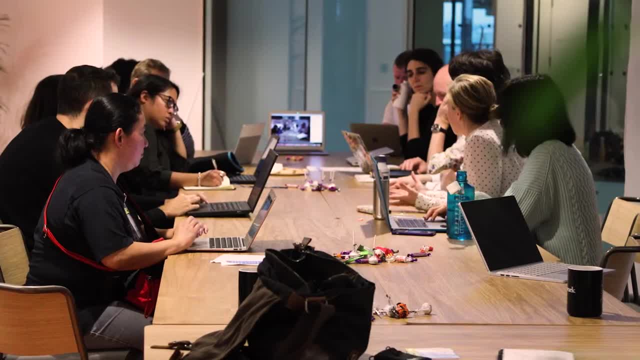 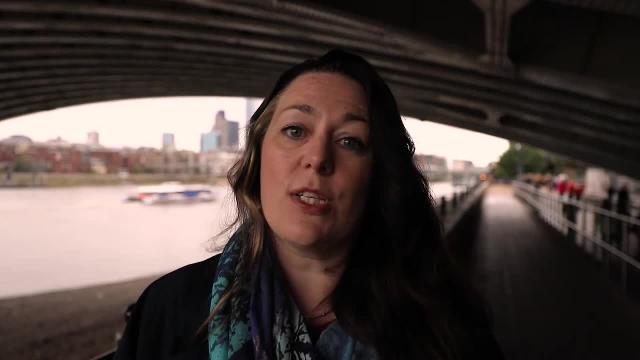 much more work to be done. We hope that this video will explain a little bit about what our charity and the individuals, communities and organisations that we work with have done over the last few years towards closing the gender gap, and also to encourage others like you to get. 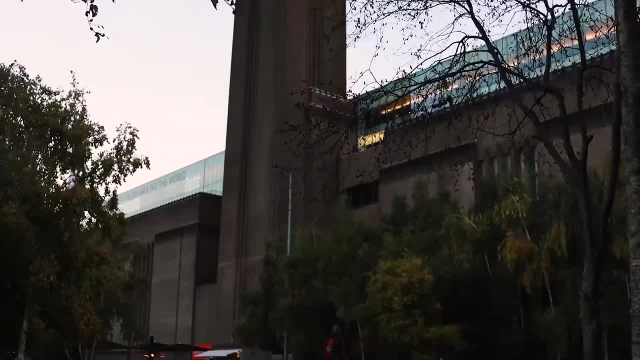 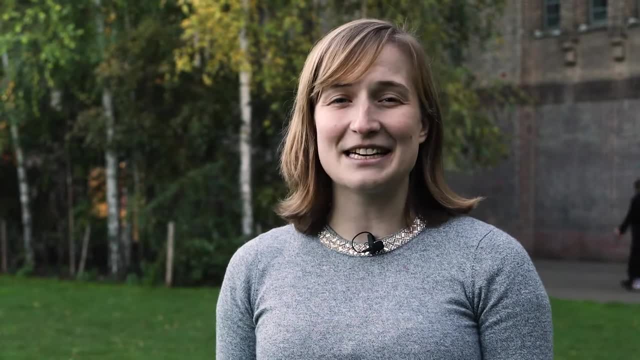 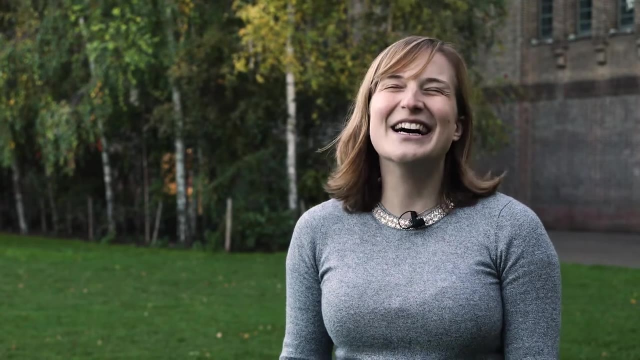 involved. I'm Alice White and I am a digital content editor at Welcome Collection, and I'm also their Wikimedian in residence. I think the main thing that's changed in the time that I've been doing this role is how many people are approaching us to do things, and I started out speaking to people and 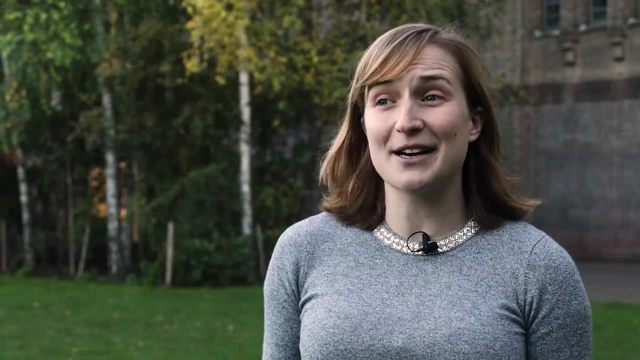 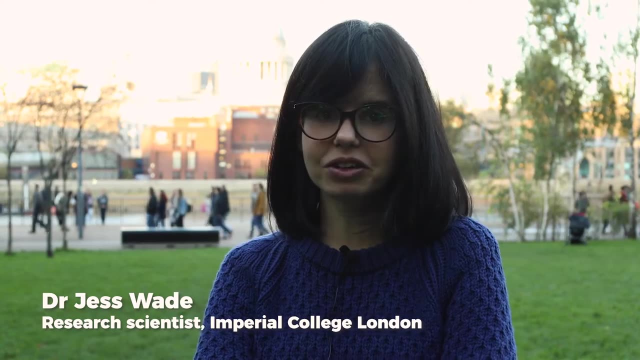 inviting them to participate. and now people are hearing about this wiki stuff and thinking that sounds amazing. I want to do that and approaching me. My name is Jess and I'm a physicist at Imperial College London. Alice taught me not only about how to edit Wikipedia, but 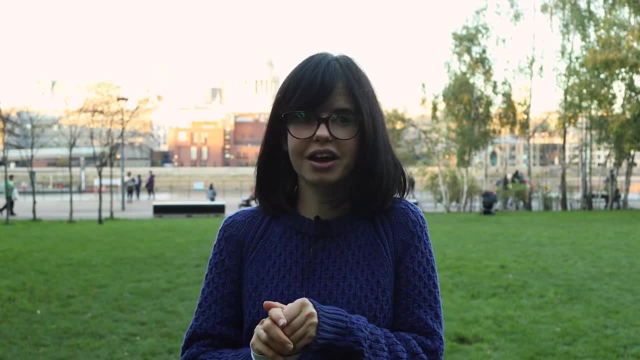 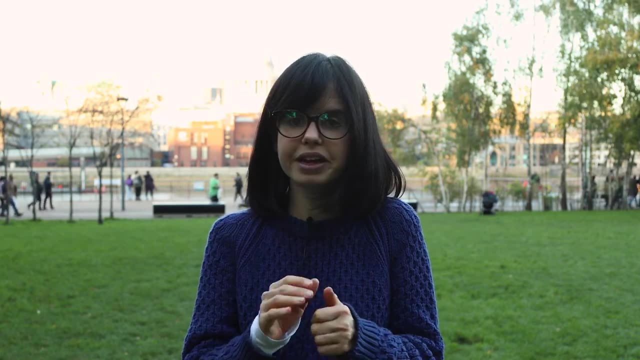 also about the horrific gender imbalance on the website and I for a few months just thought, hey, this is kind of cool, I'll talk about it a bit. and then realised, kind of over Christmas and New Year at the beginning of 2018, that actually to change things properly, I'd have to really invest some time into it. 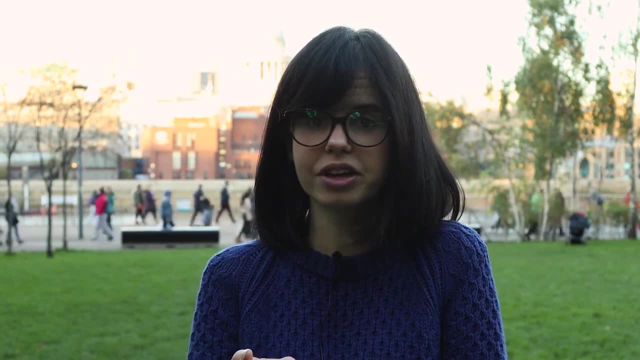 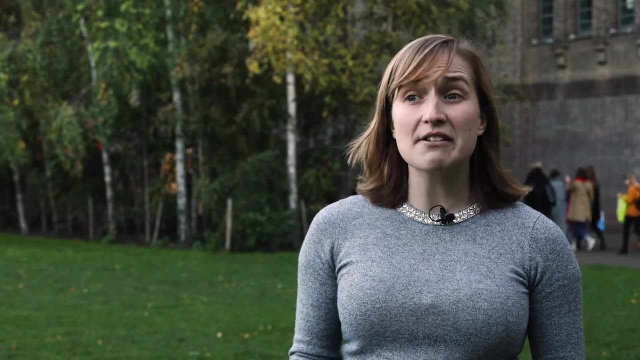 so I decided I'd make one page about a woman, scientist or engineer. every day, People want to see how they can make a positive change. so it's all very well to run an event that starts out very, very doom and gloom. and here is this huge problem, and it's insurmountable. but what has the most? 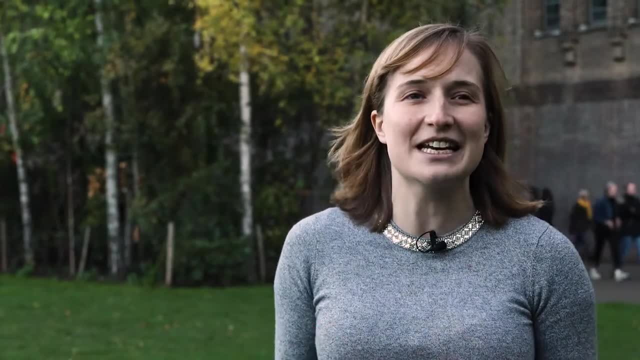 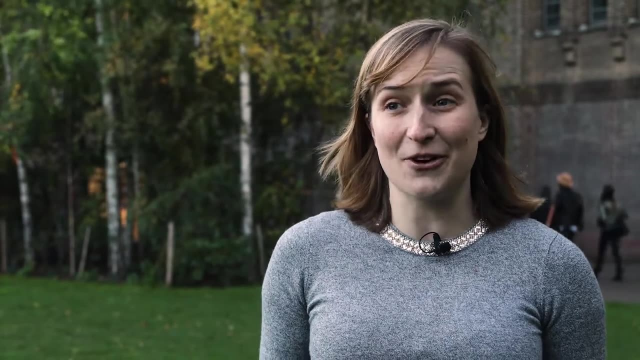 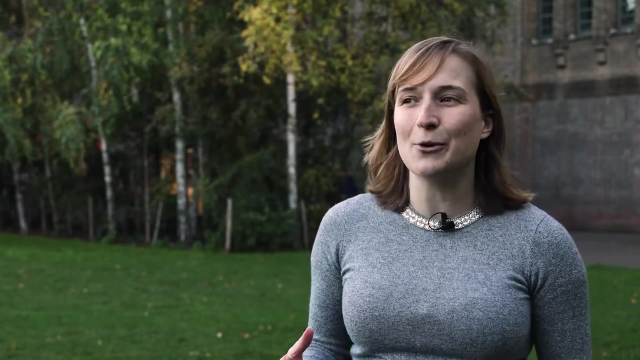 successful outcome in terms of motivating people and getting them editing is, I think, the way that we communicate that Wikipedia is a collaborative, volunteer-led project and you can do something about that and talking to them about the progress that's being made and the opportunities for them to make a contribution to the project. 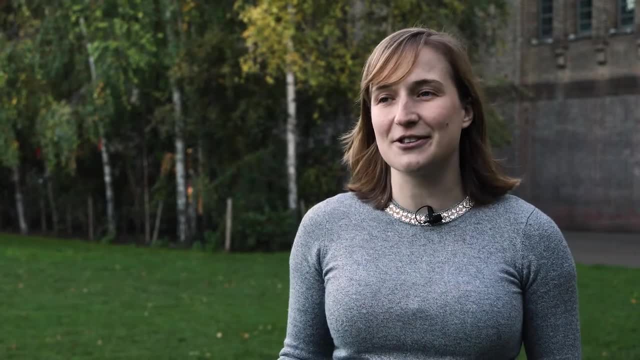 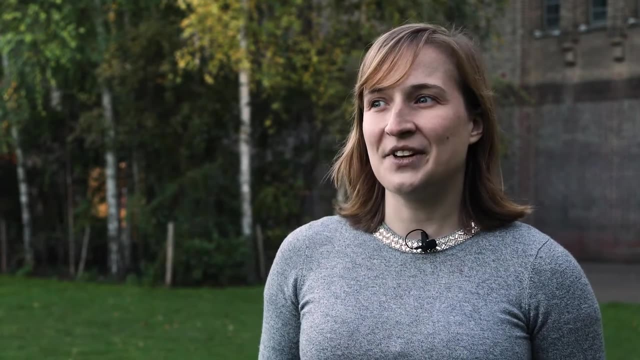 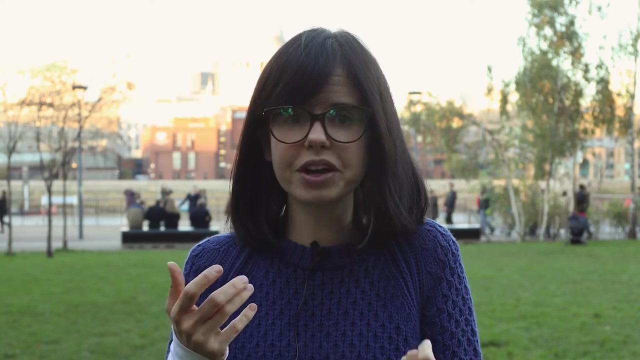 The contribution, big or small, whatever they have time for, and I think inspiring people with what they can do rather than making them feel sad about how things are, seems to have worked really, really well for us. and then someone from the Guardian wrote an article about it in the summer- actually a physicist who used to be at Imperial 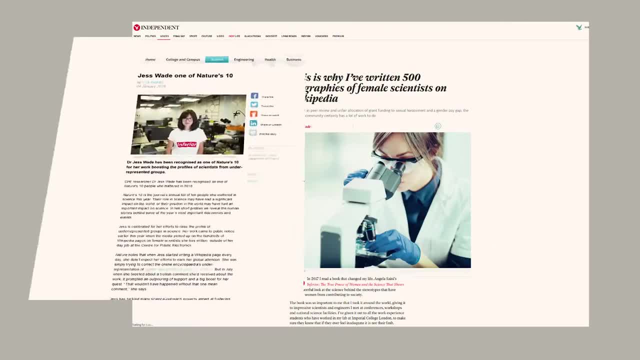 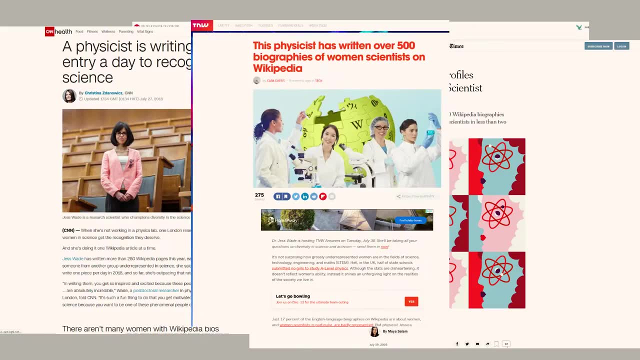 called Hannah Devlin wrote an article about it in the summer and after that now it's gone pretty crazy and I feel like a lot more people are reading the pages that I create and also making their own pages, and I feel a bit of a responsibility to make my pages better and better and better now. so, yeah, it has. 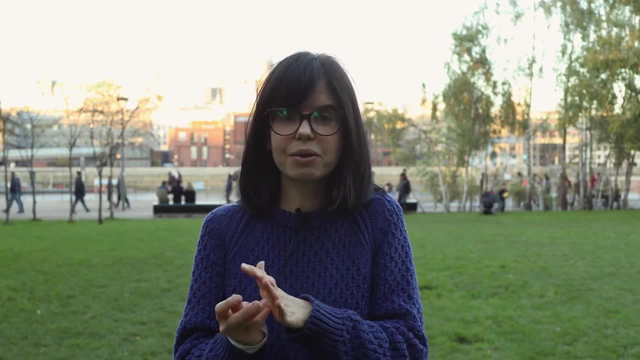 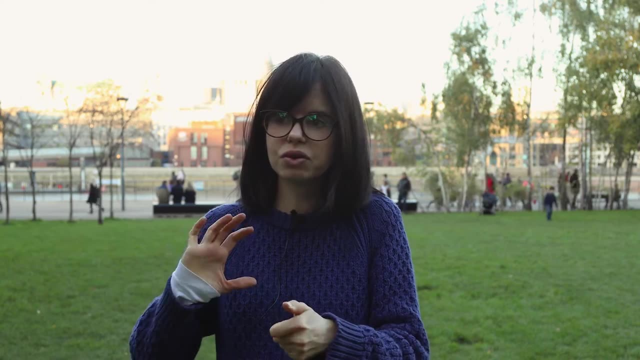 definitely snowballed in recent months. It started a discussion about how we celebrate and recognize the women scientists and engineers who are already working in science, and I think that's one of the biggest challenges we have. it's not just all about the inspiration, it's not just about putting role models. 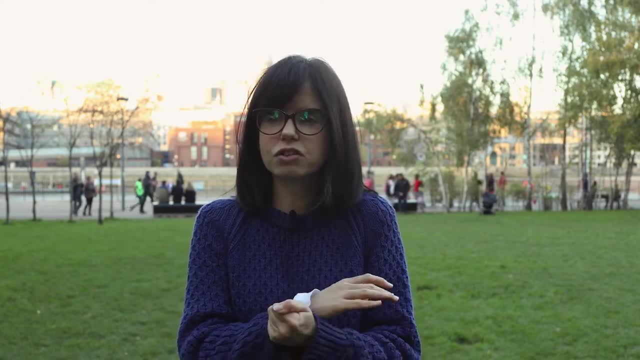 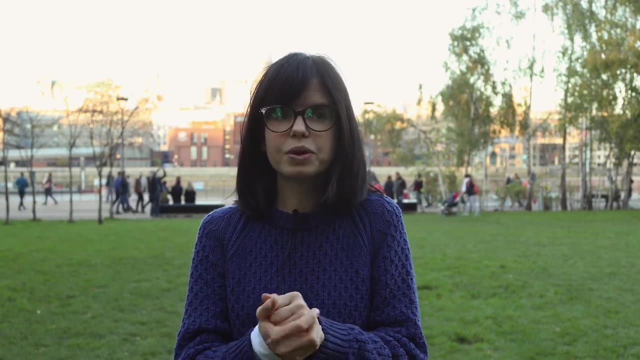 there for young kids to see. it's also about recognizing there are so many phenomenal women, people from underrepresented groups, working to better understand and promote their work. We need to protect our planet and we don't recognize and celebrate them enough, and if we don't, we'll just lose them, and we need to do a better job in. 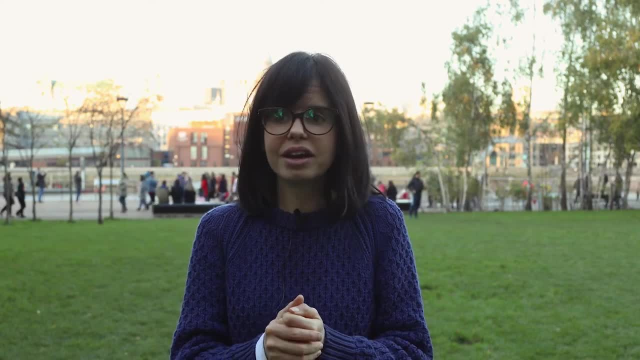 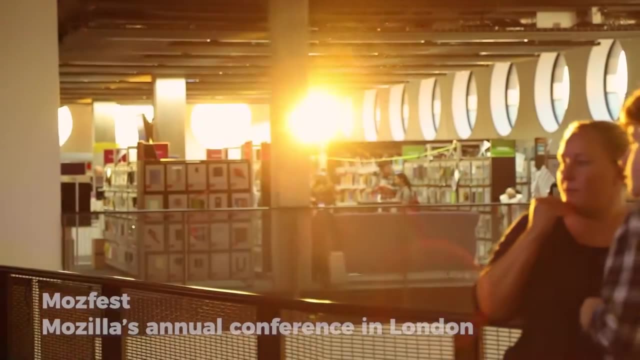 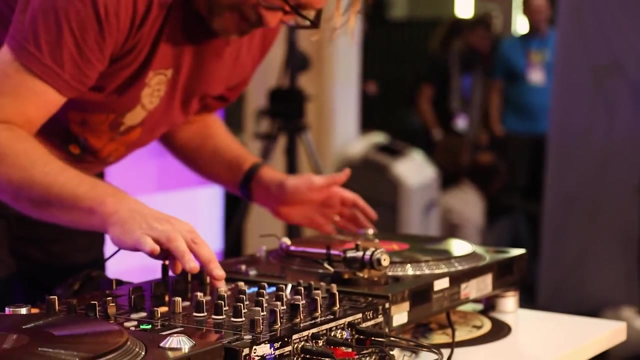 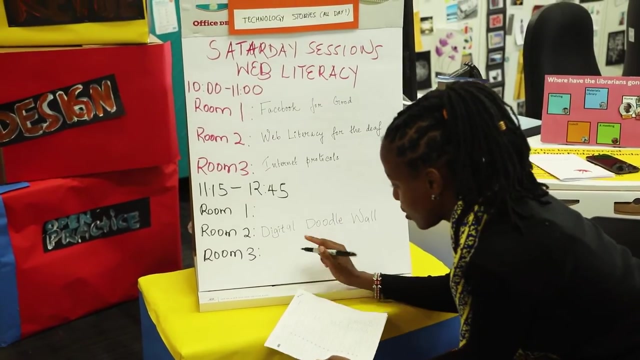 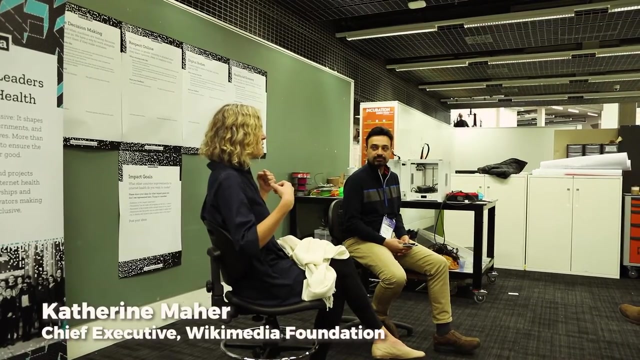 science of saying: you are incredible and we need to keep you here, and maybe one tiny little way we can do that is making sure that all these really phenomenal people have Wikipedia pages. It's totally fine to me that most average community members have no idea that the foundation exists, and I think that's okay. the question is: what can we? 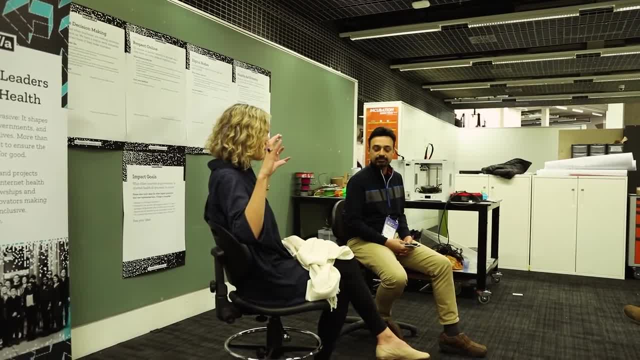 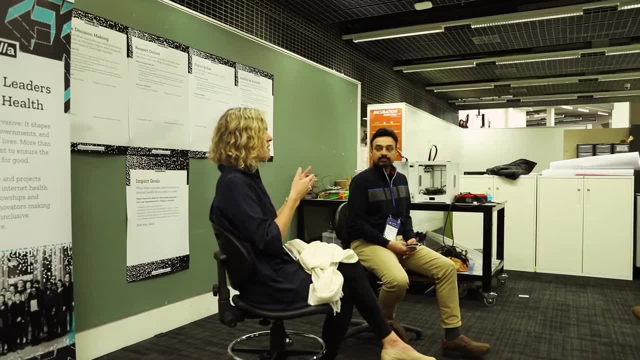 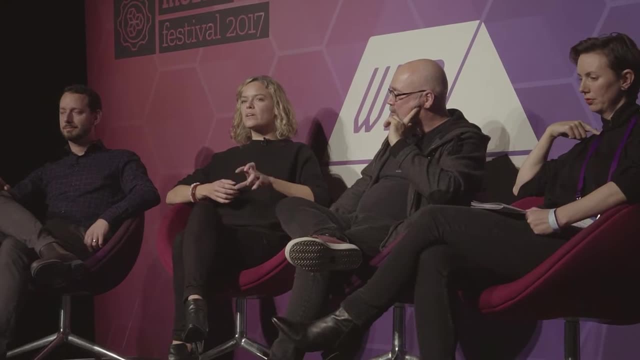 do as the foundation to ensure that that community becomes more representative or more inclusive or what-have-you, without necessarily needing to get to the level of the person who's adding a citation at the end of a sentence. We actually, we actually started talking about equity as a major value of ours, and I think that what's 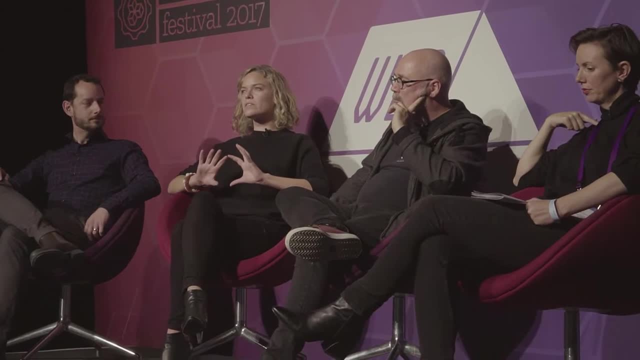 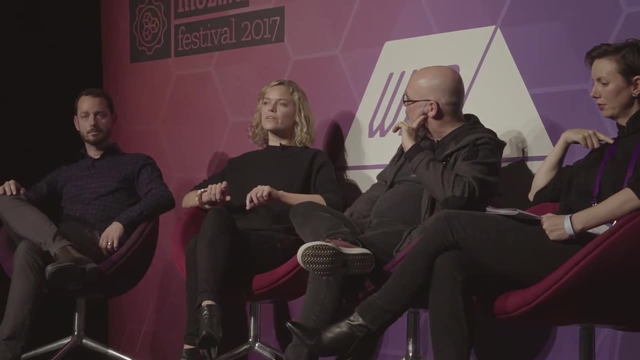 interesting- and it sort of speaks to Ryan's point- is that we can media. for us, the vision statement is a world in which every single human can freely share in the sum of all knowledge, so that implied equity as a value is in there. it's a world-changing vision. it says nothing about an encyclopedia, but you know and I 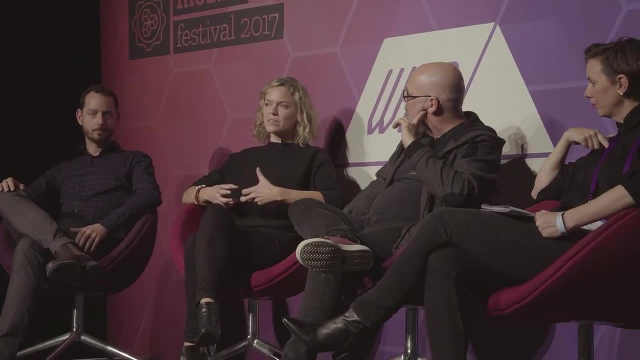 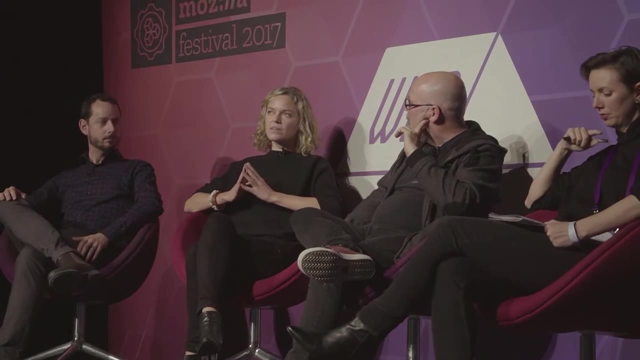 think that we were quite radical when we started and in some sense and embraced that radicalness, and then we got comfortable and now I think we have to be radical again if we're going to get anywhere near What that sort of that call is for us to achieve. 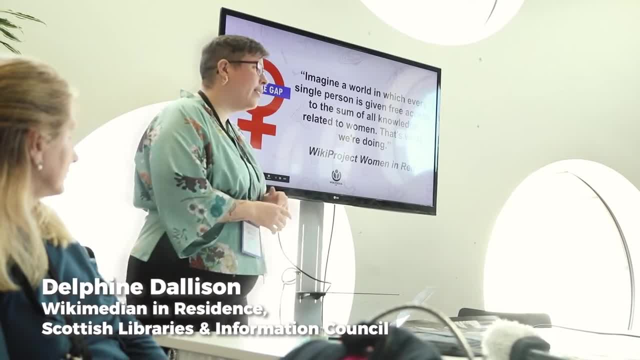 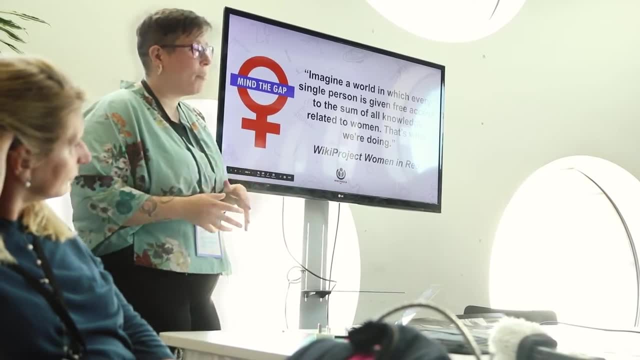 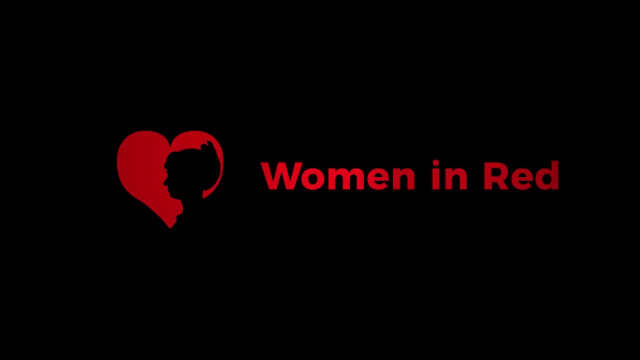 Every month, the wiki project Women in Red issued new lists of names for every country across the world, and editors spend their time actually trying to fill that gap. My name is Roger Bamkin. I became involved with Wikipedia one year after I was 20.. I was not part of the 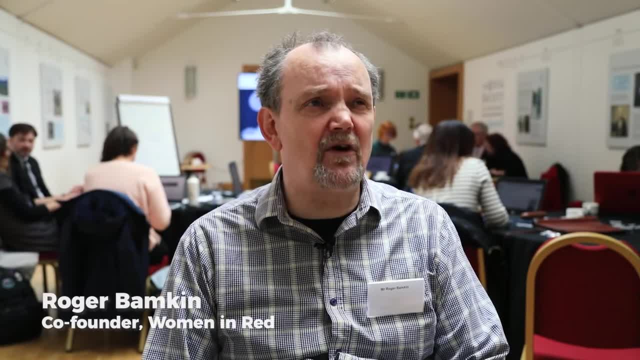 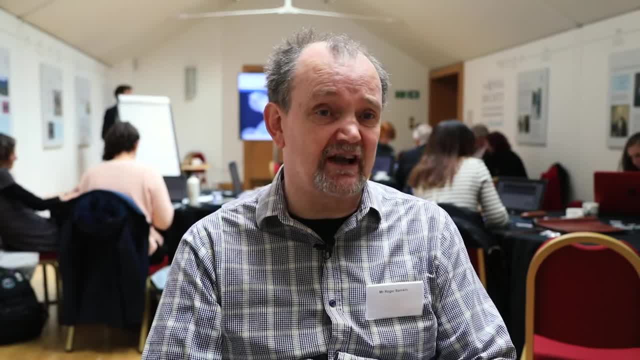 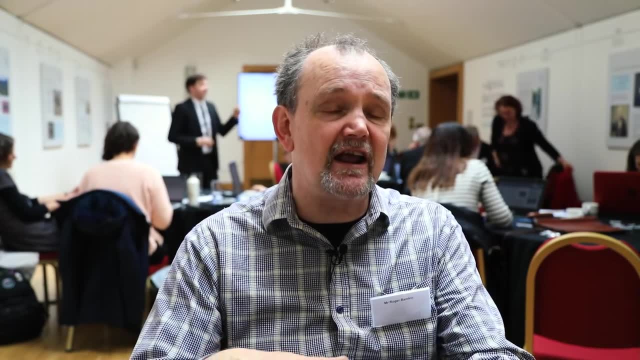 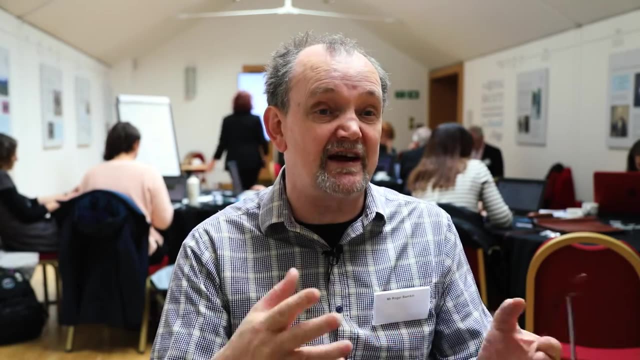 my children were editing it and they went. this would be interesting. At the time, Wikimedia had this idea that if only they could increase the number of women on Wikipedia, then that would fix the problem, because they saw the fact that there was nine out of ten editors were. 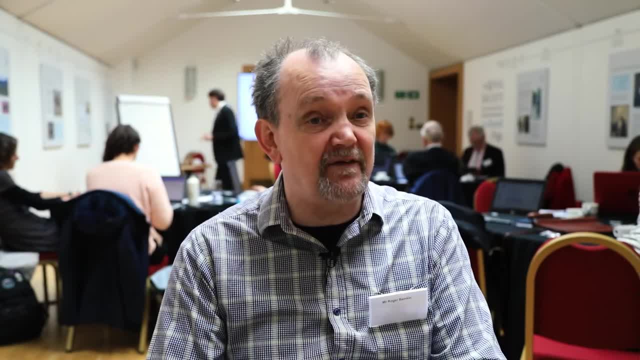 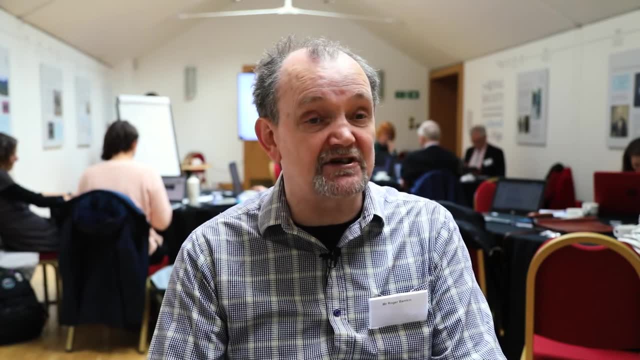 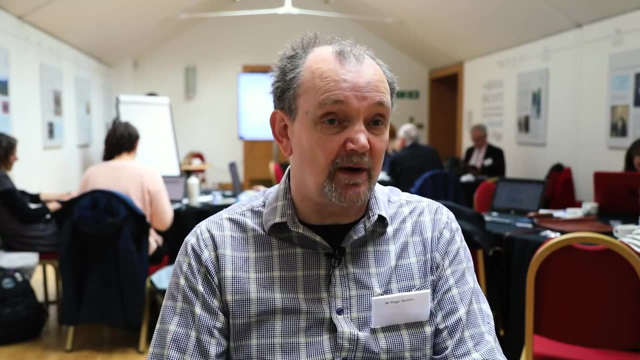 men as the problem. So in 2015 there was a Wikimania conference in Mexico and I wrote a proposal to say we ought to establish a project that would get not just women but people of all genders to solve this problem and try and have an equal number of men and women on Wikipedia. Fortunately, a good 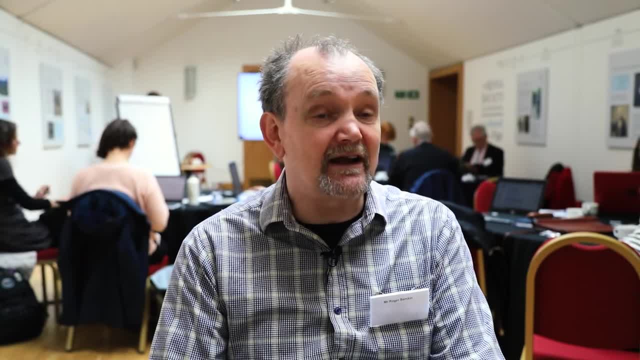 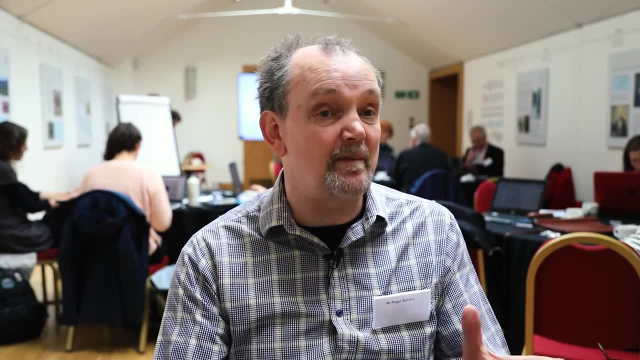 friend of mine, now a lady called Rosie Step, came forward and said she would be a joint founder with us of the project, and that was how the proposal was given in Mexico And after that we thought it would be a good idea to start a project in Mexico. So we started a project in Mexico and after that we thought we 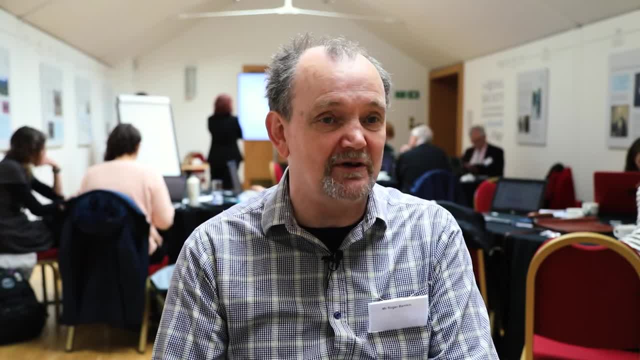 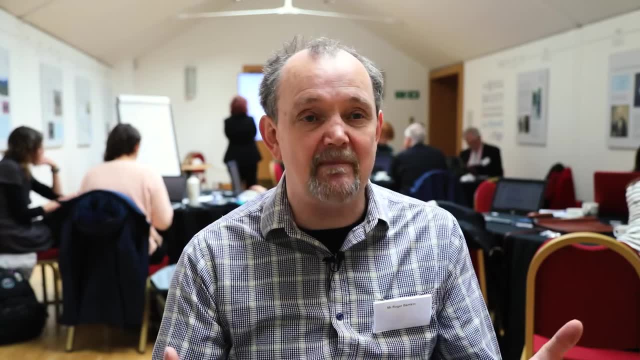 thought we'd have 15 minutes a frame, We thought it'd be an Andy Warhol moment and that would be the end of it, But it gathered an awful lot of people. Wikidata was suddenly the key to it, because suddenly we could measure things like gender and 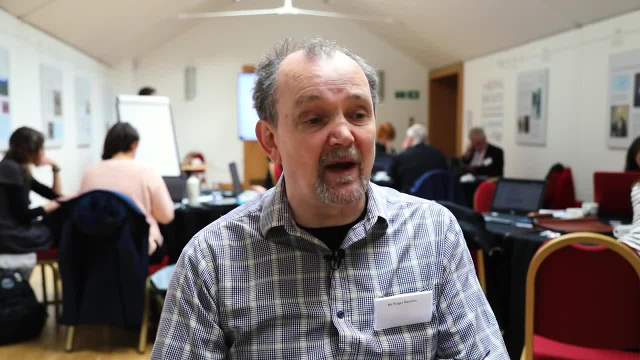 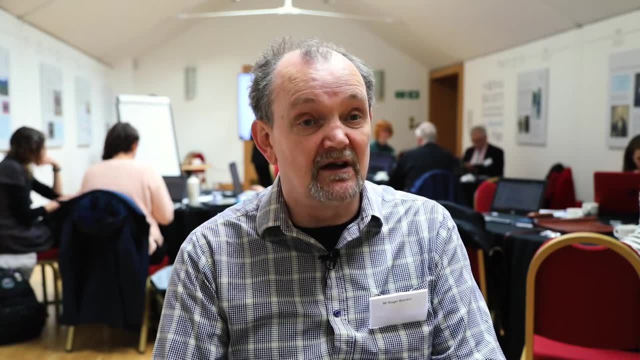 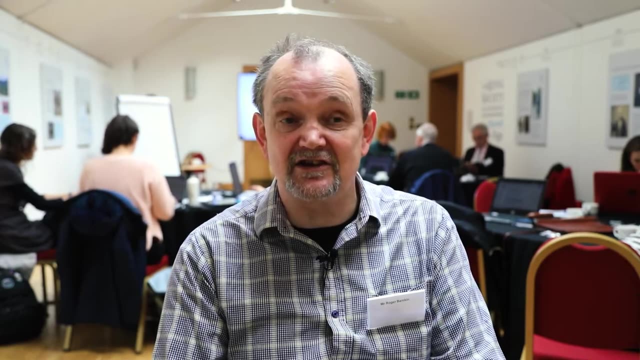 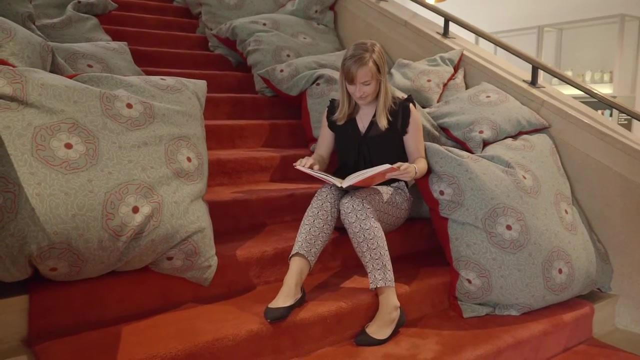 since then we've gone to. we believe there's been about 82,000 articles created. We are working in 22 different languages. The editing seems to go on 24 hours a day. It's just stunning. So Wikipedia is a great way of making people visible online and easily. 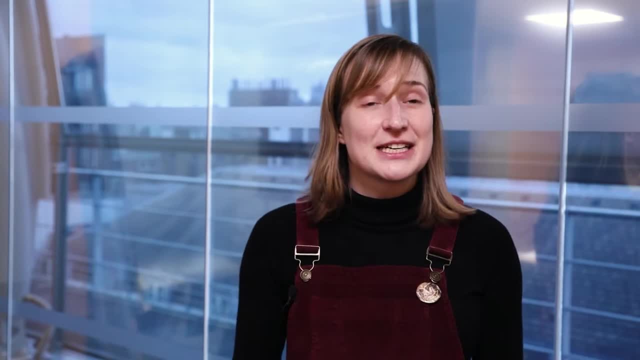 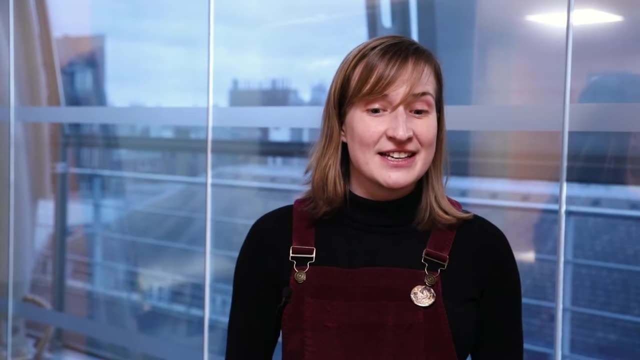 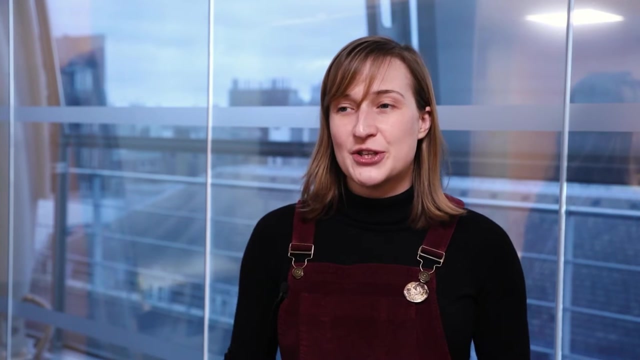 findable to other people who might like to then do more research and find out more about them and amplify those stories. So I had one person come along to Wikifilm that we ran and she said she really wanted to create a page for this particular woman engineer who was fascinating and she had a really 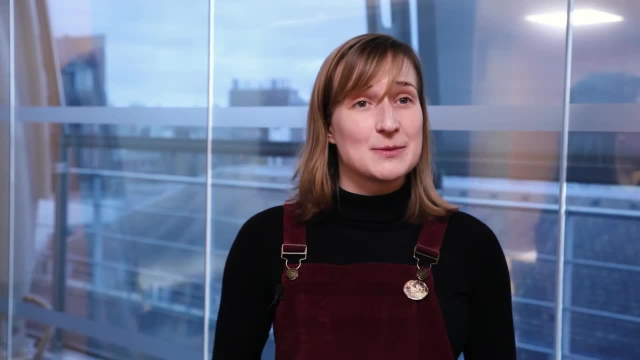 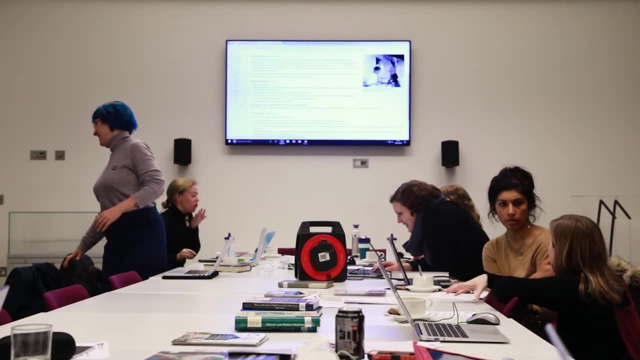 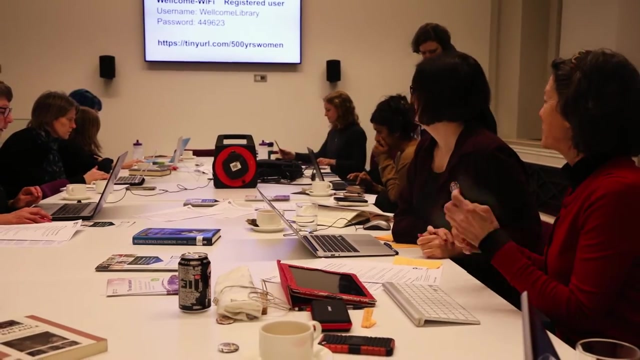 interesting and varied career, but there weren't very many accessible pieces of information about her. All of these fascinating details were buried in publications that weren't really available online. So this woman who came along to one of my my editing sessions created a page for her inspirational 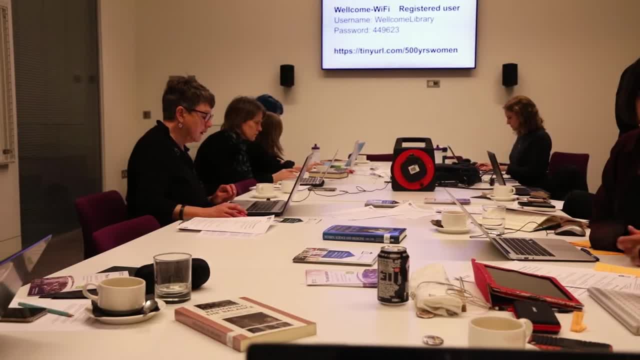 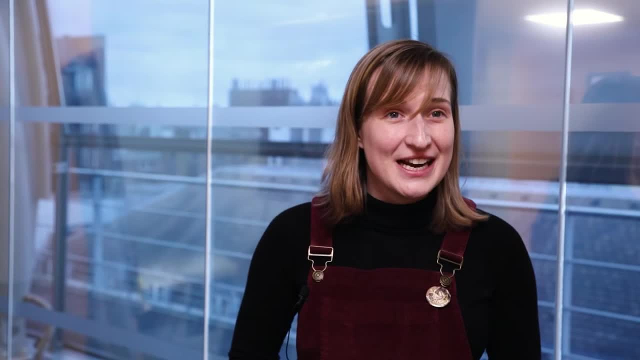 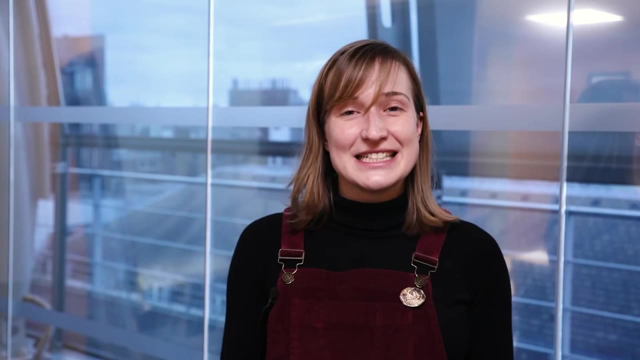 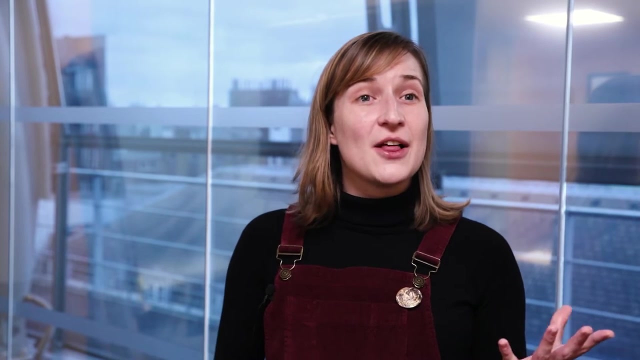 woman engineer who she thought needed better recognition, and after creating this Wikipedia page, she approached a radio show And pitched a segment about this woman and how fascinating she was and that shows. researchers were then able to very easily and quickly find information about this woman, And I can't definitely say for certain that the Wikipedia page is the reason. 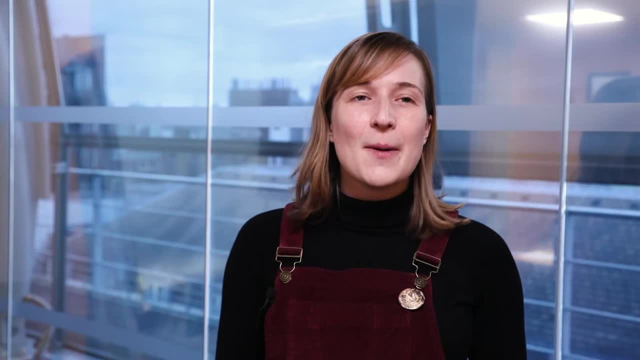 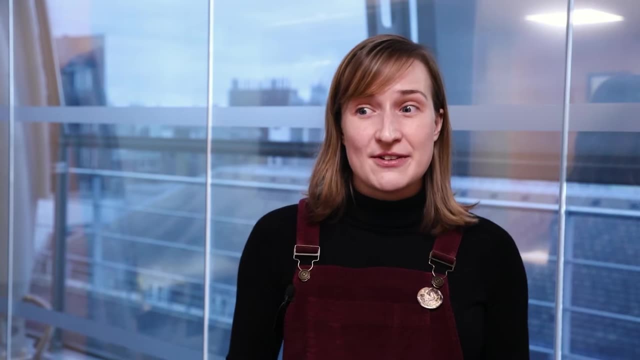 why the show did actually get commissioned, But I think it. you know, the woman herself said to me: I know researchers and I know how time pressed they are when they're involved in making these kinds of shows And it definitely helps to make the 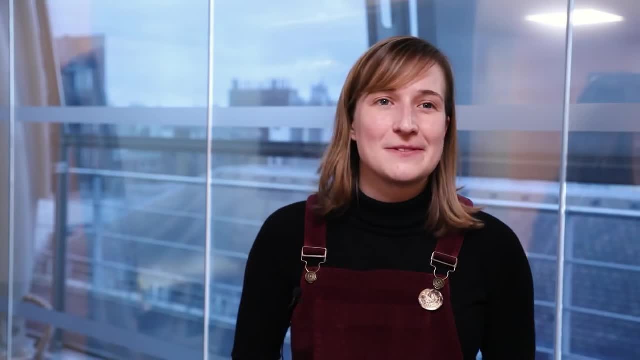 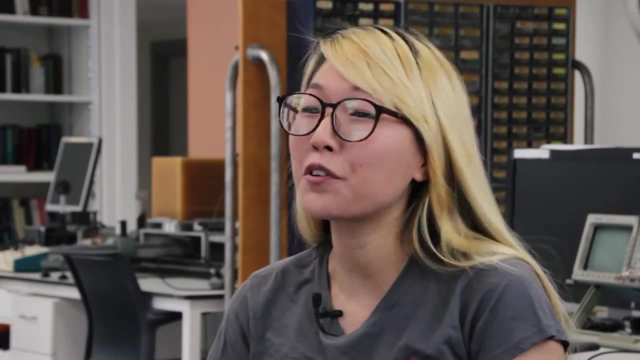 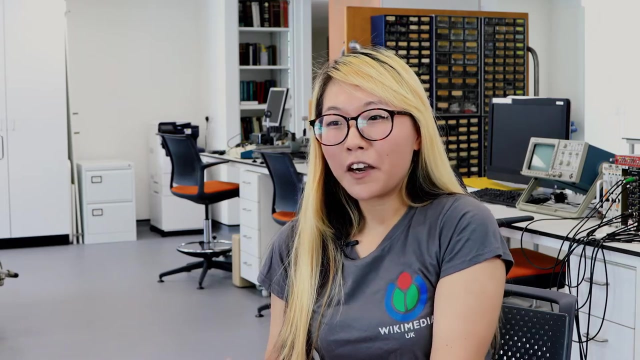 stories as easy for them to find and pursue as possible. I'm Dr Ying Leah Lee. Everyone calls me Leah. I'm a physicist at University College London and what my work is is optomechanics. The way that I became more involved on Wikipedia is through Dr. 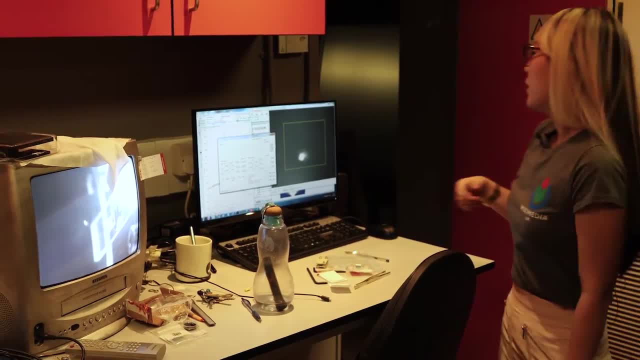 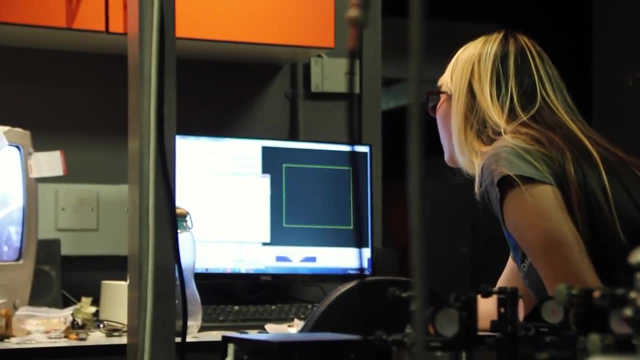 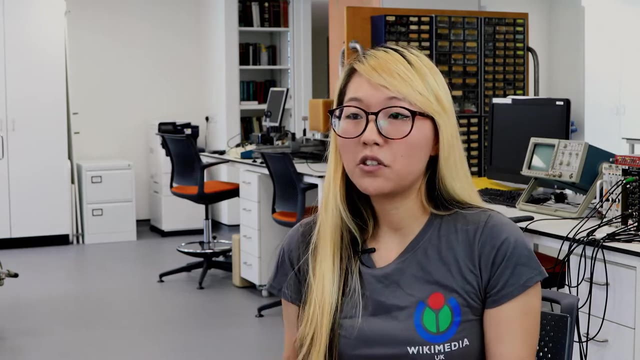 Jess Wade. She's a researcher at Imperial College. I started running the UCL women and physics group and I've been trying really hard to get more and more speakers to come and and do talks, because I think it's quite nice to kind of step out from your own problems or your own situation. I got. 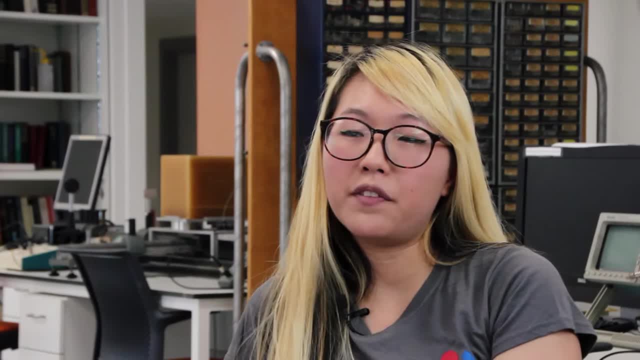 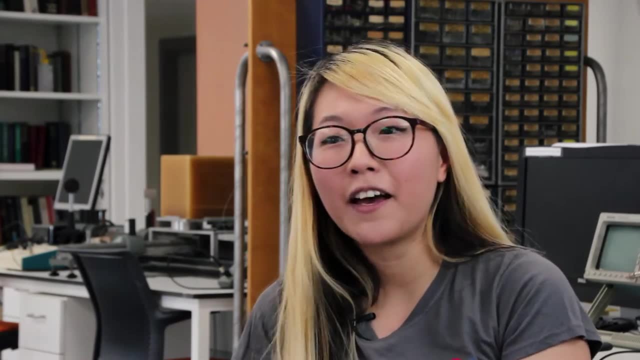 in touch with Jess because I really wanted her to come and and talk about everything she's doing. And she said: oh yeah, sure, but why don't you come to Imperial for this wikithon that we're doing and then we can talk about it there? And I kind of thought, okay, that's interesting. I was a bit 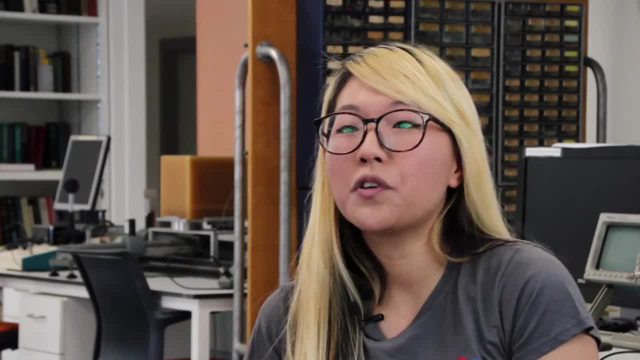 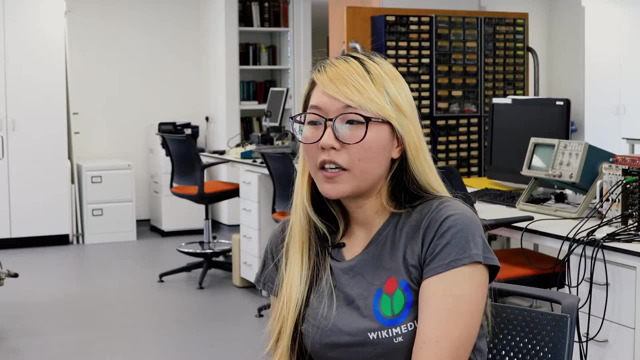 scared because I had never actually edited anything on Wikipedia before then. But she said she said that her and Alice White from the Wellcome Trust they were going to do all the training. there's nothing to be afraid of. I kind of came out of that with a whole new impression of what 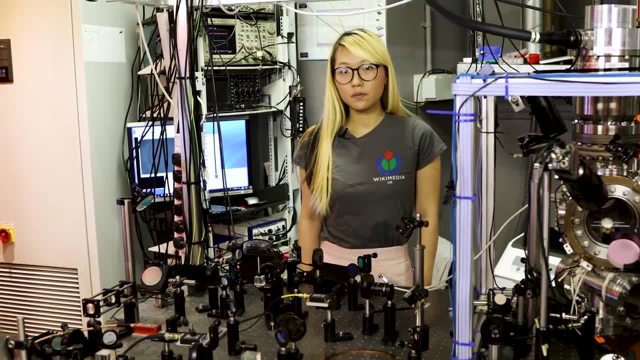 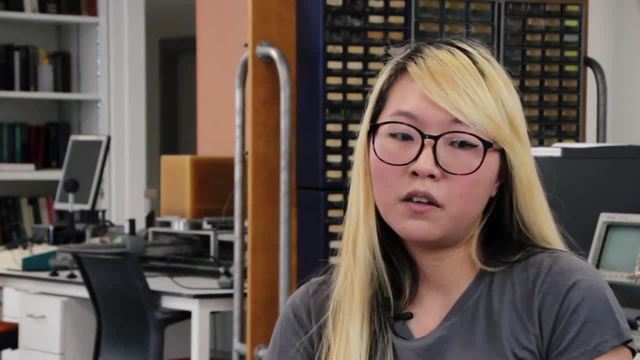 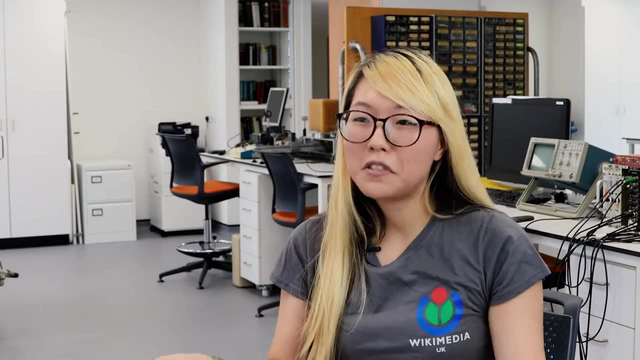 you can do with Wikipedia to make a difference, Instead of trying to get individuals to come and talk to- you know 20 or so people at UCL. with Wikipedia, when you make a biography about a really prominent female scientist, you're impacting them, but you're also contributing. 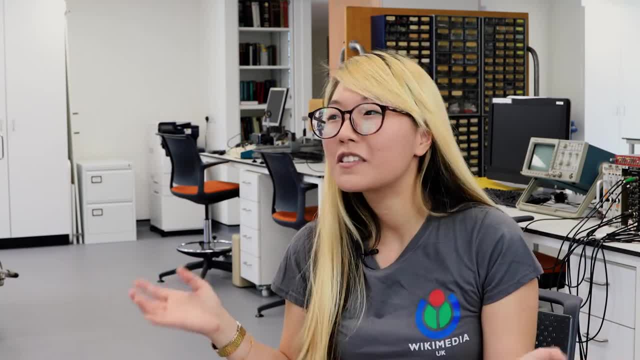 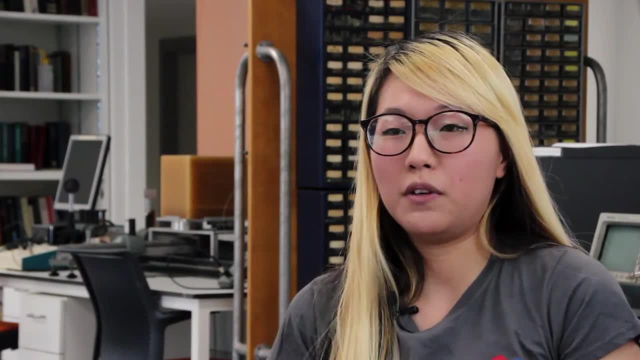 to like the future of the science And that's what I've been doing for the last couple of years- The historical record of kind of science for like the whole world, And so that was really empowering because I couldn't have thought of anything else I could do here that would. 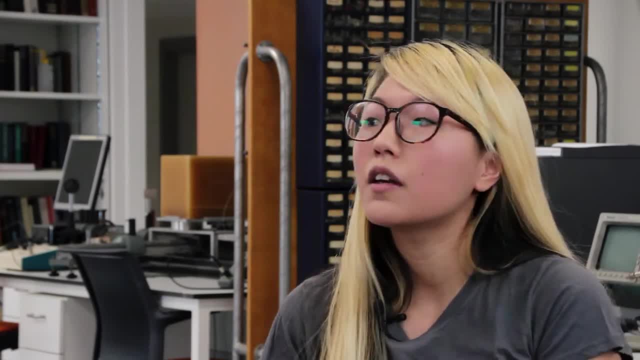 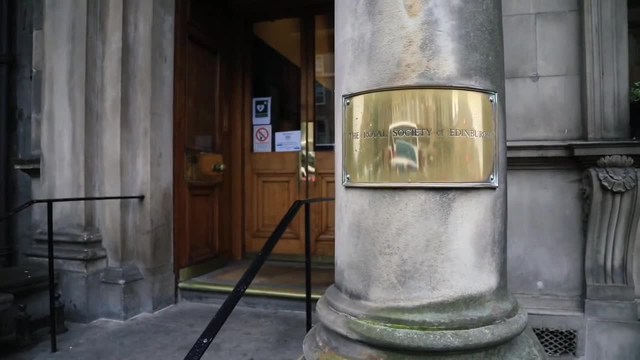 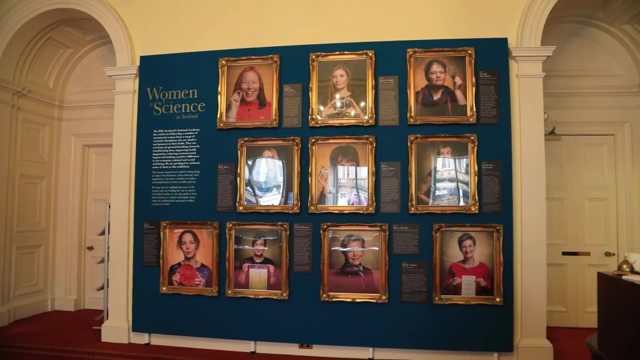 have that much of a impact outside of Justice University. Wikipedia has gaps. We know that Wikipedia has gaps. We have structural bias in society, so we end up with structural bias on Wikipedia And one of the things that we do at Wikimedia UK is to try and encourage people to fill those gaps- One of the strategic objectives of Wikimedia UK. 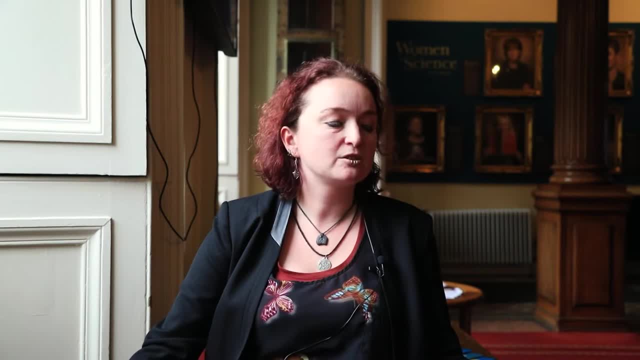 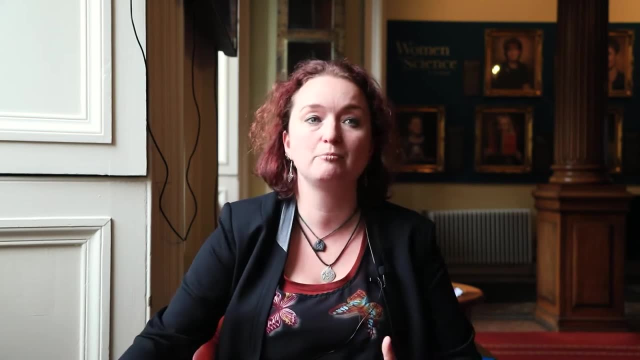 is to address underrepresented content on the encyclopedia. So one of the things that we do in Scotland- part of what I do as Scotland Programme Coordinator- is to try and encourage our partners to do work in that particular area. So we've worked in our projects with the Scottish Libraries and 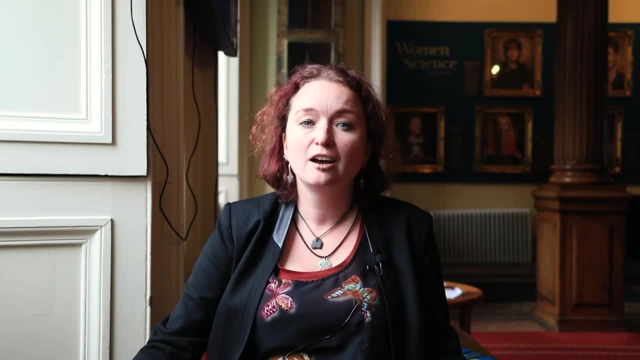 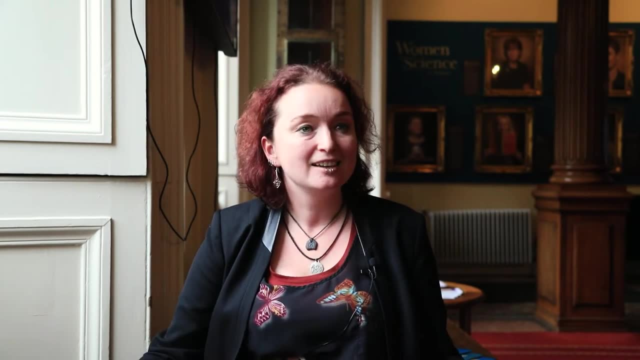 Information Council. we held an edit-a-thon on the Isle of Skye, about women of Skye, and that's about finding where those sources are bringing people together and getting them, encouraging them, to edit about those topics and to create those articles. 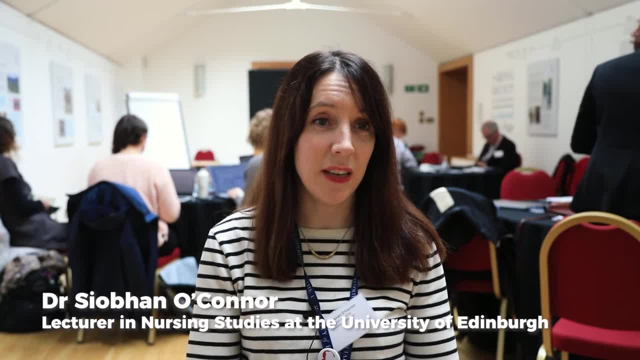 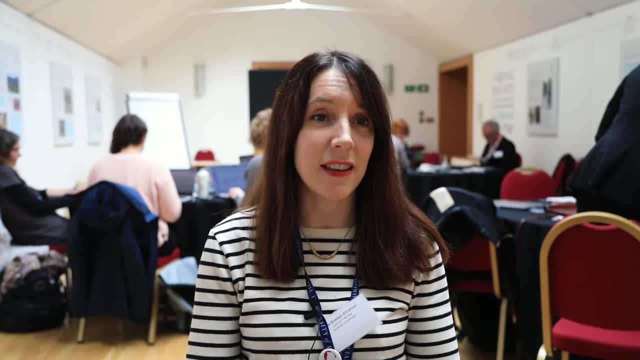 Hi, my name is Siobhan O'Connor. I'm a researcher based at the University of Edinburgh. I got involved with Wikipedia about two years ago. There was an event running an edit-a-thon running at the university where they were trying to get more nurses up on Wikipedia, So I saw that advertising. 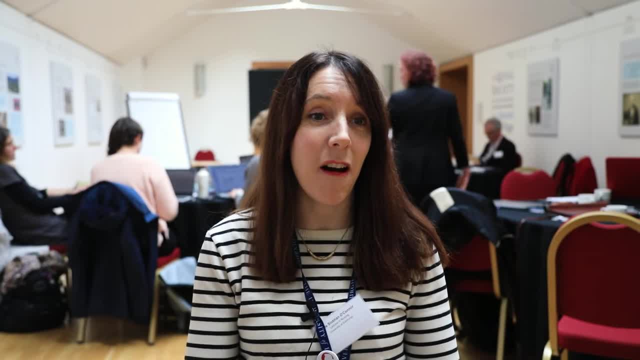 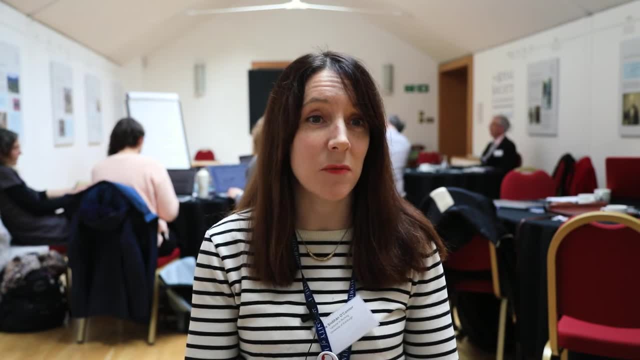 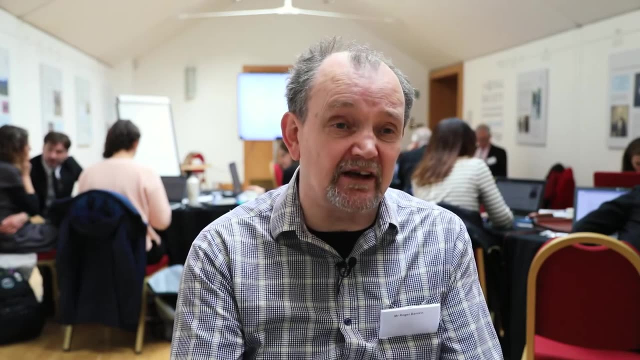 because I'm a nurse, a nursing researcher, I was really keen to go along and learn about how to create Wikipedia articles and understand a bit more about, I suppose, the gender imbalance on Wikipedia in terms of the information that's on there. As you say, we can't fix history, History is fixed. Battle of Waterloo was 99% blokes But since we've 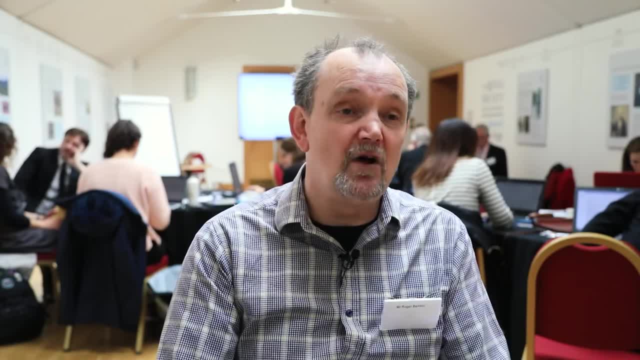 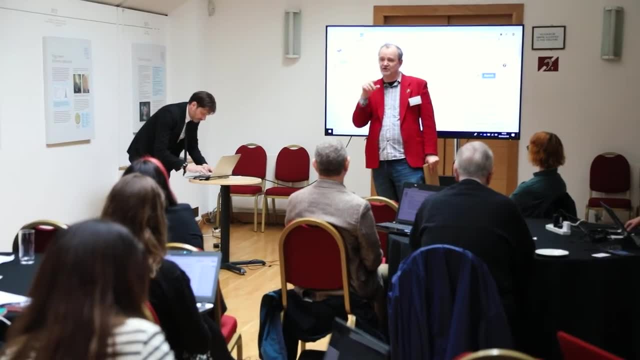 had the project, we found out that there were women. There were women working waiting in the nearby town, writing books, writing articles. We can write about those. When I was working in engineering, we used to say that a project was something that was defined with an end. 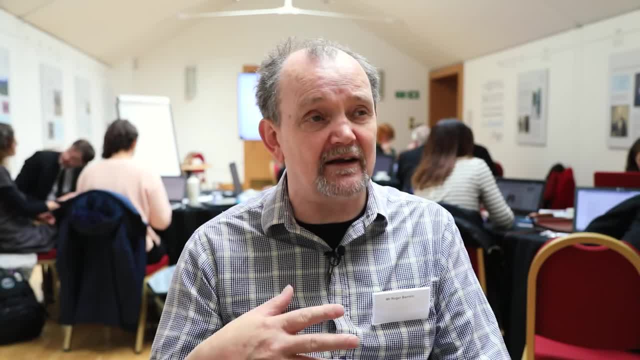 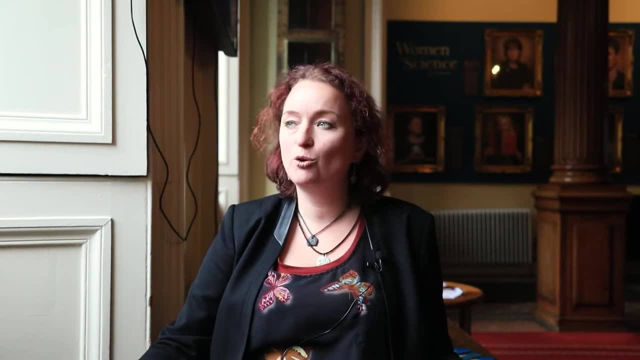 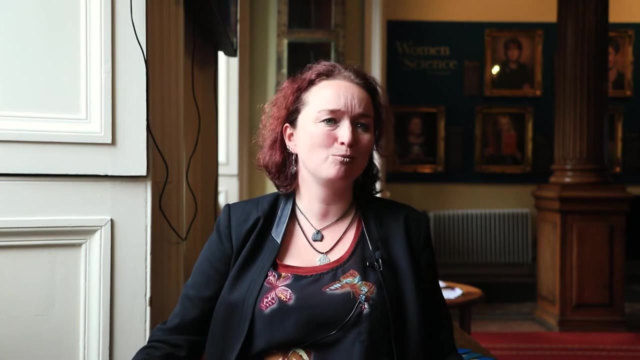 And certainly Wikipedia itself and the Women in Red project doesn't seem to have that defined end. We need more editors. We need more editors. We need people with a wide variety of interests. I want students to edit. I want professors to edit. I want school kids to edit. I want 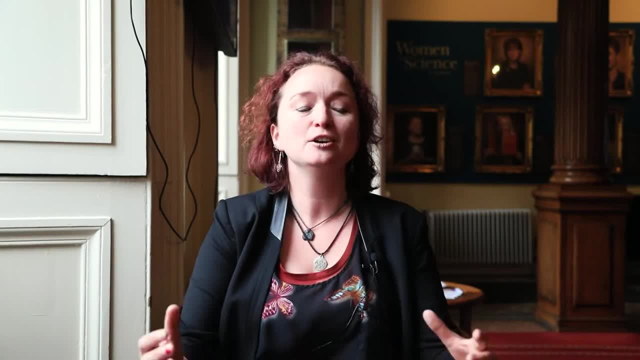 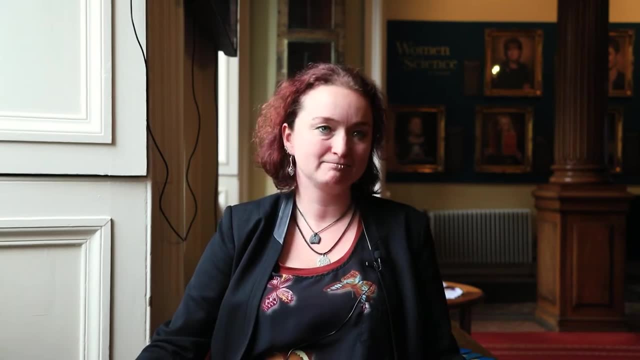 everybody to edit. I think if you have an interest in anything, Wikipedia has a niche for you, And I want more people with a wider variety of interests to get involved and get editing. I'm Robbie Lowine. I'm manager of Wales for Wikimedia UK. 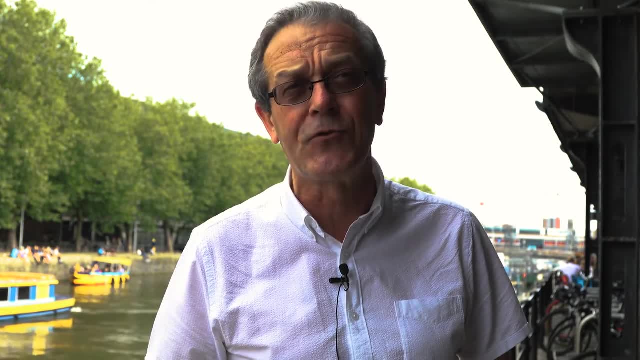 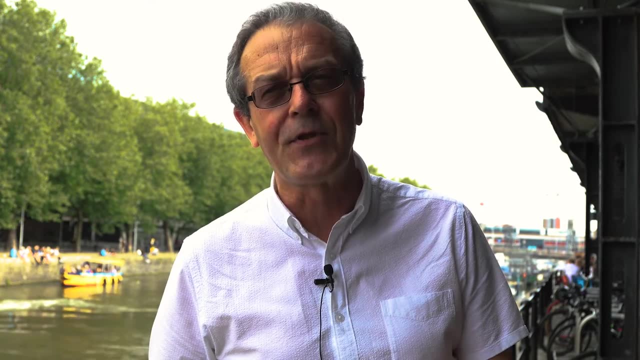 The content of the Welsh Wikipedia is excellent. We reached parity around two years ago, an equilibrium where, in fact, there are more articles in Welsh on females than there are on males, So that's a big plus. We were the first, I think, worldwide to reach that parity of gender. 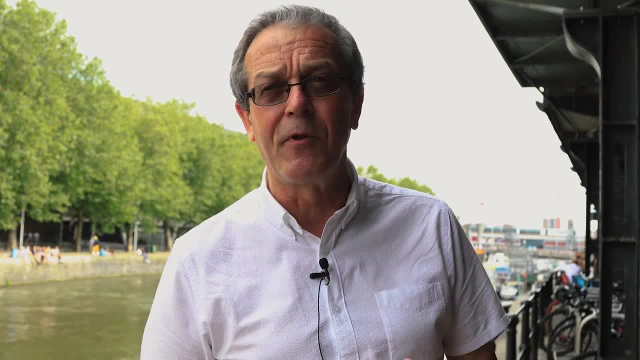 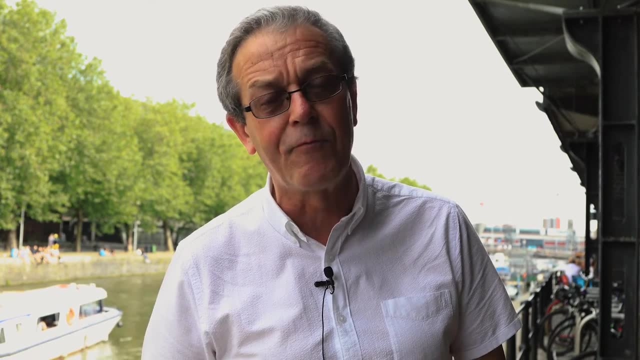 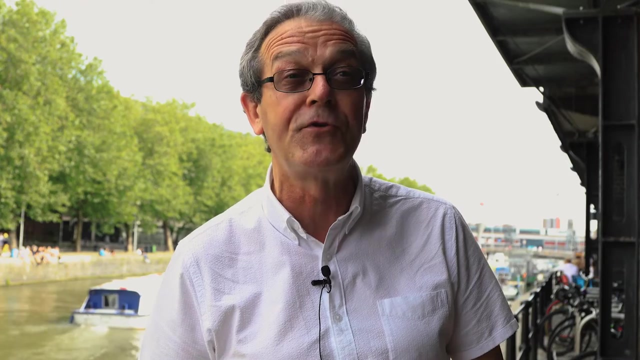 Every time we have an editathon we train people. We try to get that parity in the learners as well. Wikimorn, for example, have more female editors. We have more male editors in the Welsh Baccalaureate. They are doing the community challenge. 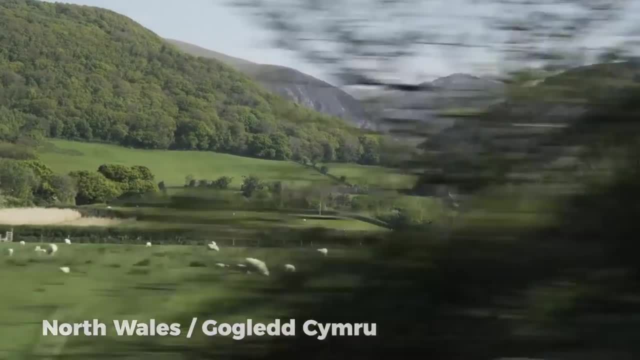 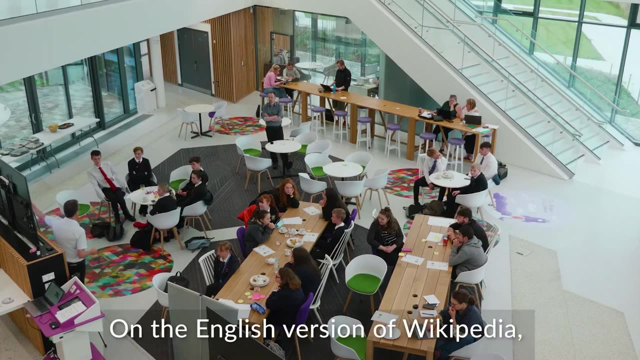 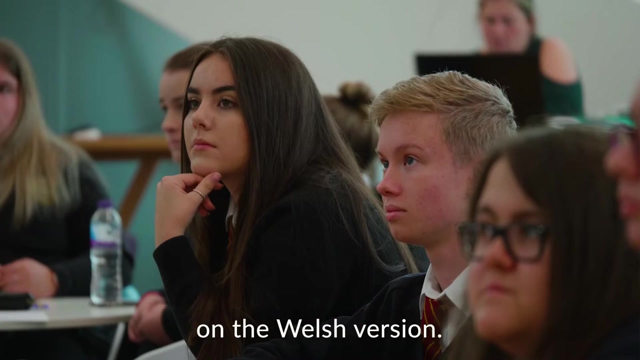 If I hold the camera, you'll get a better angle. On the English version of Wikipedia, there are more articles for women than for men, And that's why we're trying to keep the gap on the Welsh version. When I started this project four or five months ago, when I started now, there was a lot of people who were interested in the Welsh version of Wikipedia. There was a lot of people who were interested in the Welsh version of Wikipedia. There was a lot of people who were interested in the Welsh version of Wikipedia. There were a lot of people who were interested in the Welsh version of Wikipedia. 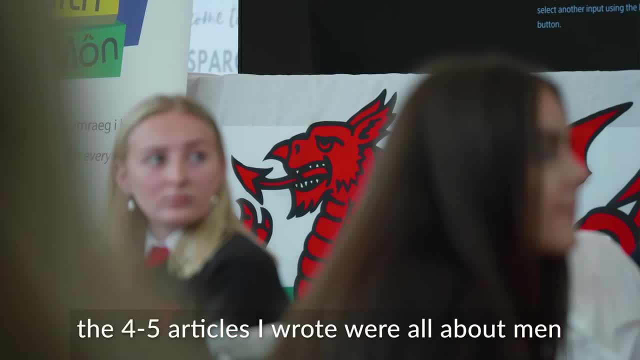 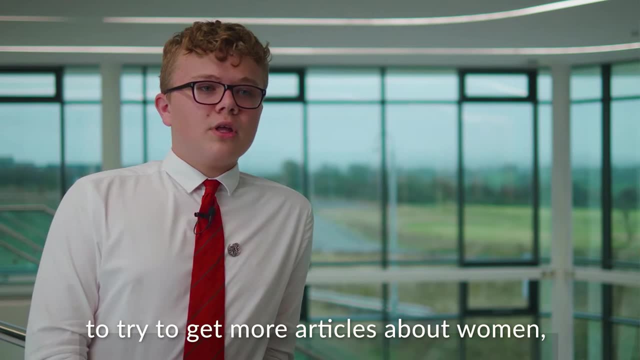 The four or five articles we've written were all about women, because we're not necessarily encouraging women to try to have more of an article about women And, as we're really coming to terms with this now, if I think about if I write an article about women for 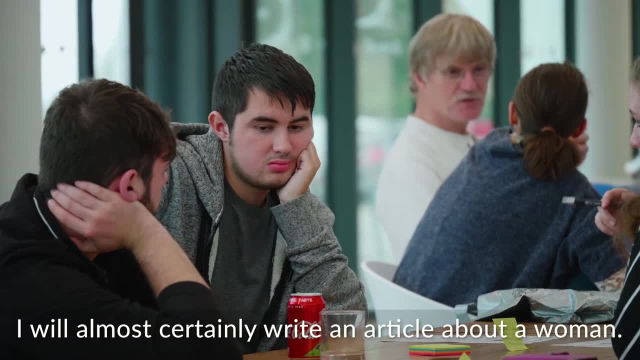 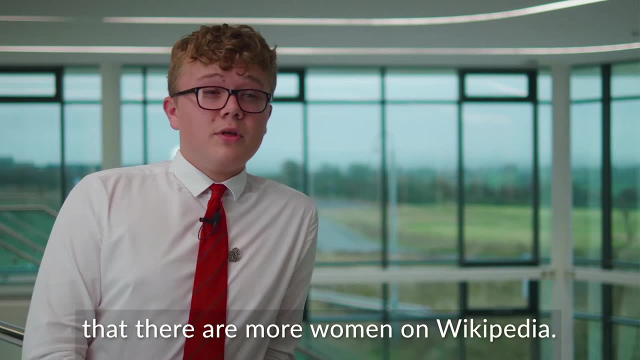 example, I'm quite sure that we're writing a book to try to have more articles about women. I think that's really positive and a really good thing too, that there are more articles now than there are on Wikipedia, So it's a good thing. 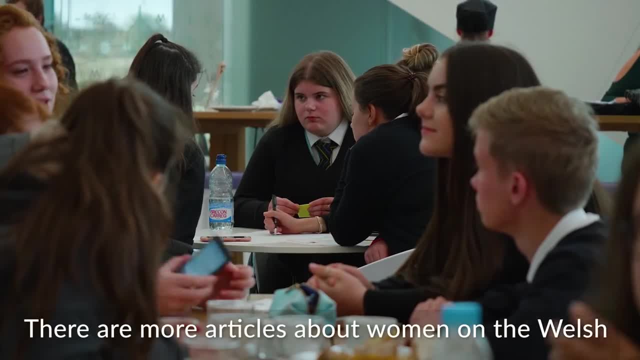 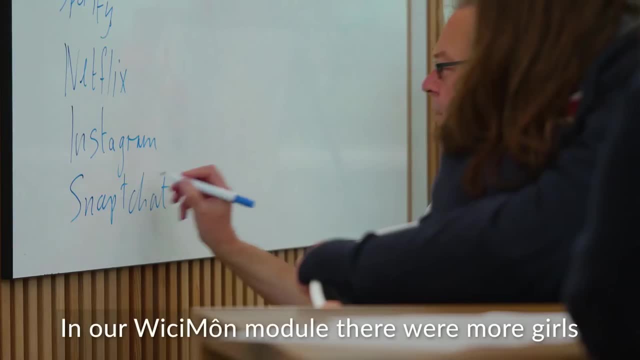 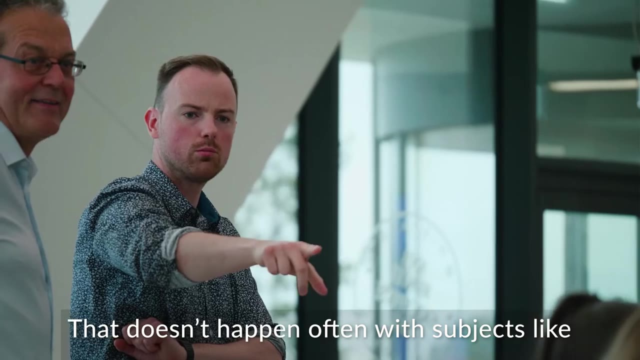 So it's a good thing. I think There are more articles about women on the Welsh version of Wikipedia and we're very proud of that. Our discussion with Wikimon was more about women than about women In the discussion. that doesn't happen a lot with things like technology and information. 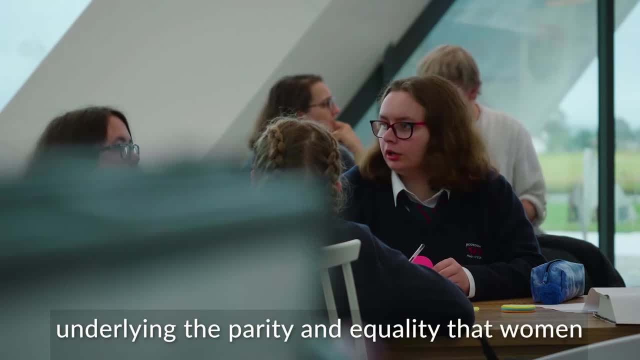 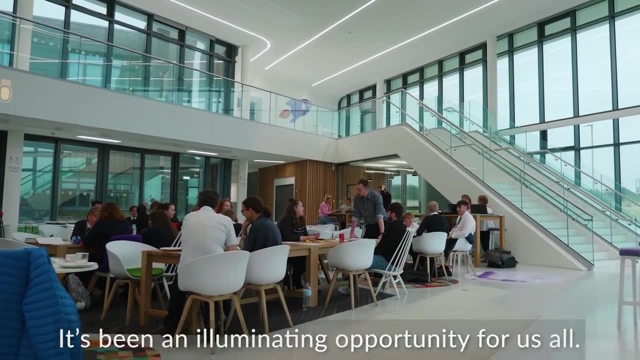 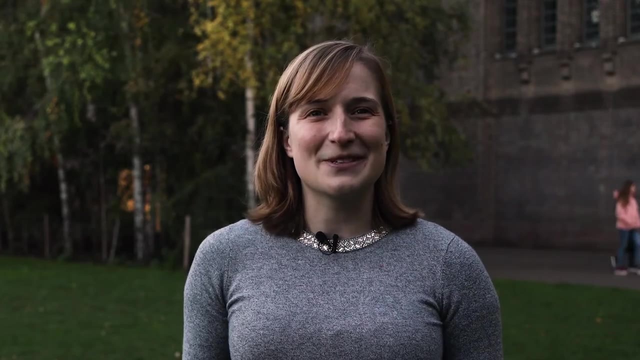 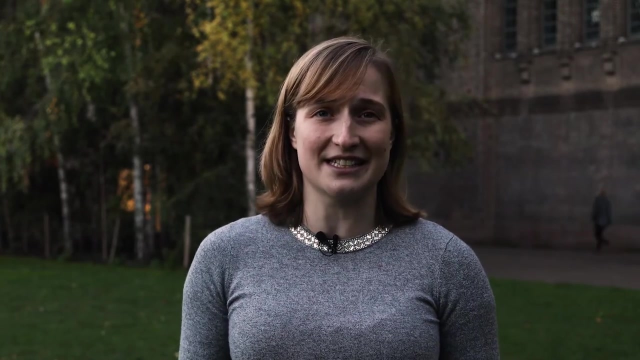 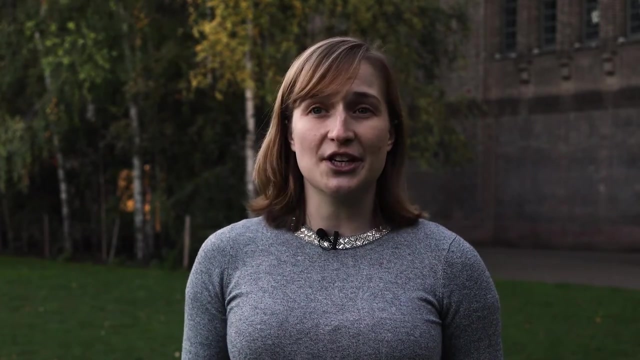 I'd like to thank Wikimon and Wikipedia for giving the focus that women are important to them and that there's no bias in the way they speak. It's a good thing, isn't it? Getting people to sign up to come along to events or getting people engaged with editing. 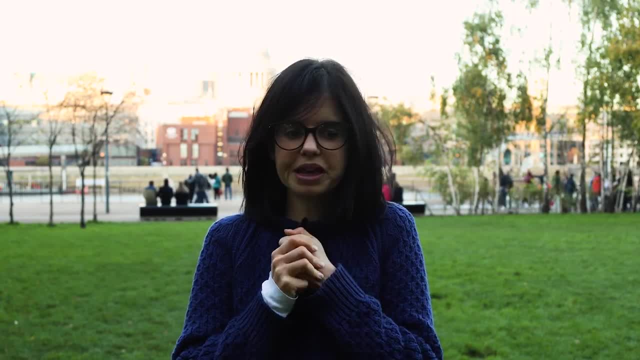 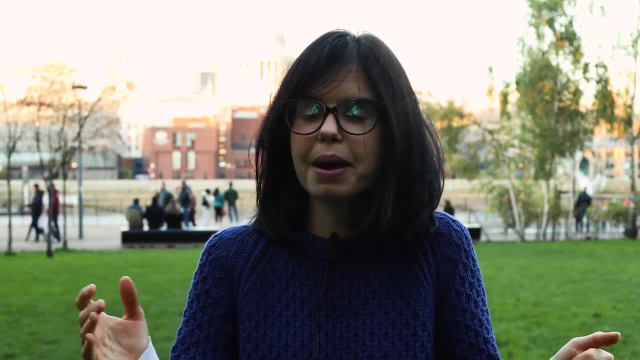 generally, because it's the kind of activity that doesn't require you to be a master of extrovert. You can feel comfortable and you can learn how to edit Wikipedia and you can genuinely contribute to a website that will be seen by millions, of millions of people every day. 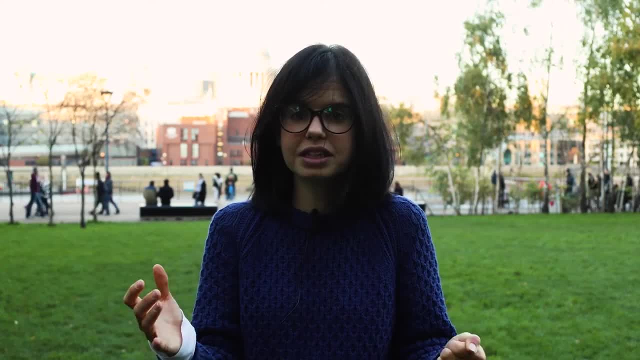 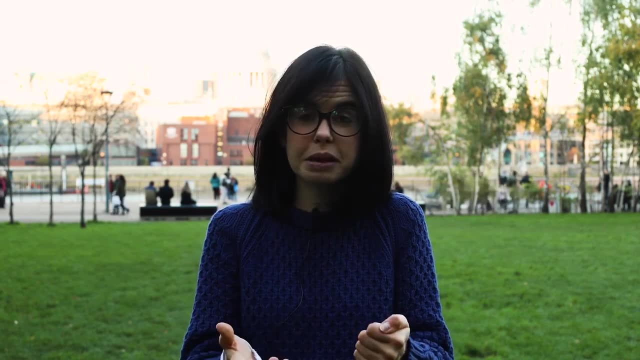 They're better protecting our historic legacy right. In years to come, textbooks will be out of date. People will turn to this for their source of information, and we therefore have a responsibility to make sure that that's as impartial as it can be. 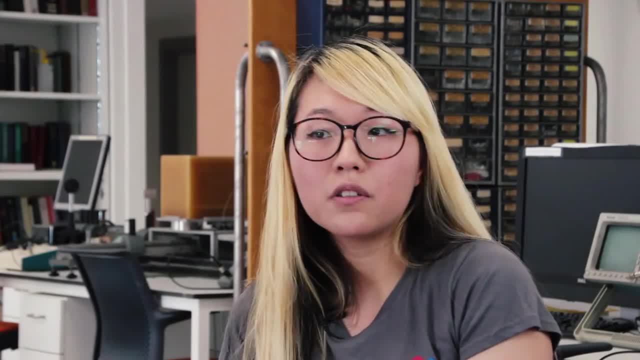 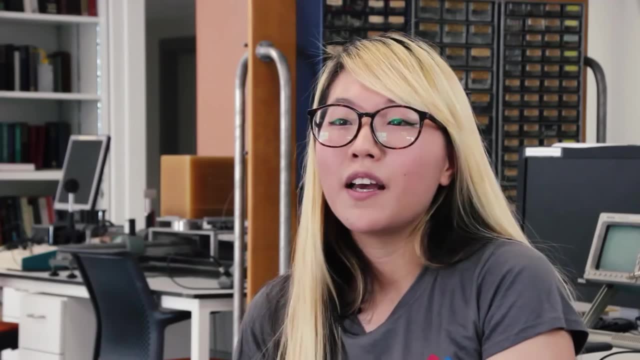 You know, it's a good thing. You can make one article and that's fantastic, but, as we know, there is something like 17% of biographies are about women, and so there is always something more that can be done. But I just find it really. it makes me happy.